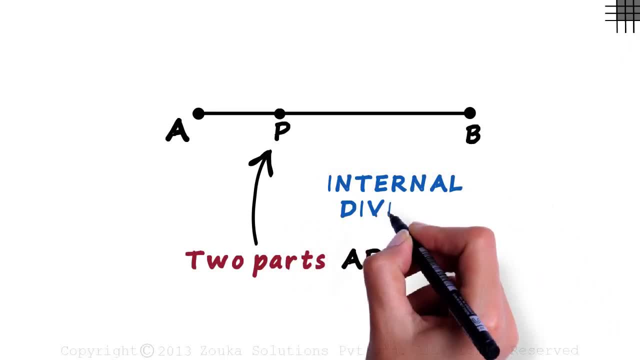 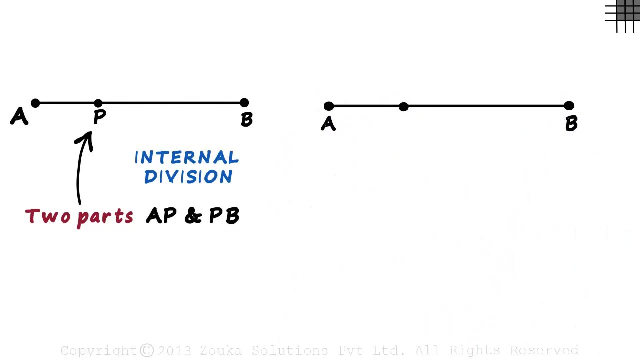 This is called the internal division of a line segment. The point P divides the segment AB internally into two parts. Can a point divide a line externally from outside? Sounds weird, but yes, it can. We see that in another video. Let me redraw the same diagram, but this time we look at a few more details. 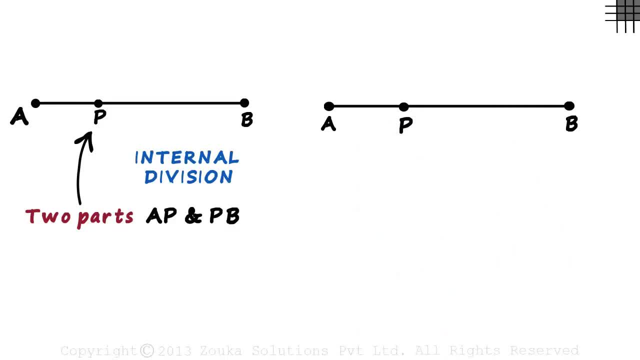 Let us assume that the point P divides the segment AB in the ratio m is to n. If this segment is drawn on a graph paper, all points will have some coordinates. Let's assume that point A has coordinates: x1 is the x coordinate and y1 is the y coordinate. 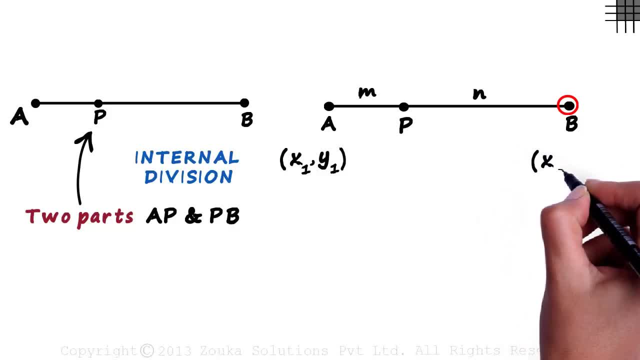 And assume point B has coordinates. What we would be really interested in is the coordinates of point P. given the coordinates of these two points, Let the coordinates of point P be. We have the coordinates of points A and B and we have the ratio in which the point P divides the line segment AB. 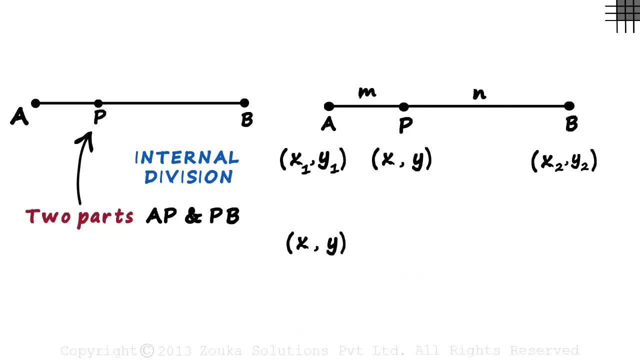 We have to find using all the information we have. So this is how the internal division formula goes. Looks really complicated at first, but in actual fact it is very simple. The x coordinate of point P equals m multiplied by x2, which is the x coordinate of point B. 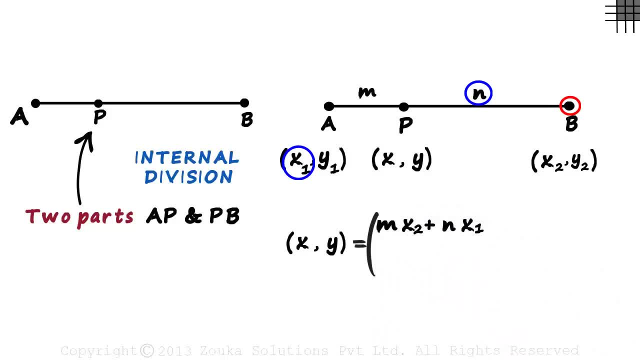 plus n, multiplied by x1, the x coordinate of point A, And we divide this entire thing by the sum of m and n, What we just found out is the x coordinate of point P. It is this multiplied by the x coordinate of this point. 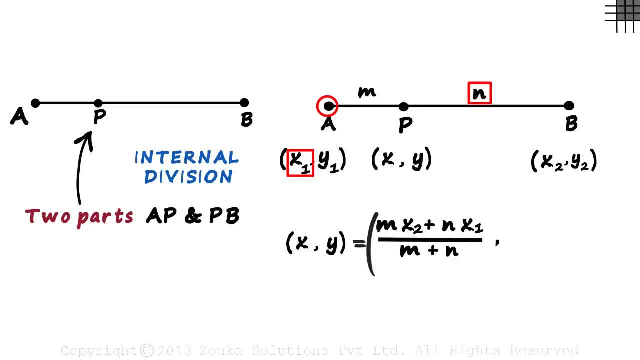 and this multiplied by the x coordinate of this point, divided by the sum of m and n. Similarly, the y coordinate will equal m multiplied by y2, the y coordinate of this point, plus n multiplied by y1, the y coordinate of this point. 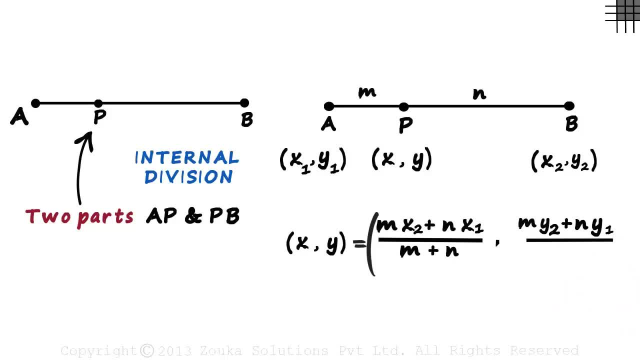 And just as we did for the x coordinate, we divide the whole thing by the sum of m and n. We go cross out here: this multiplied by this plus this multiplied by this, divided by the sum of m and n, This is called the section formula for internal division.